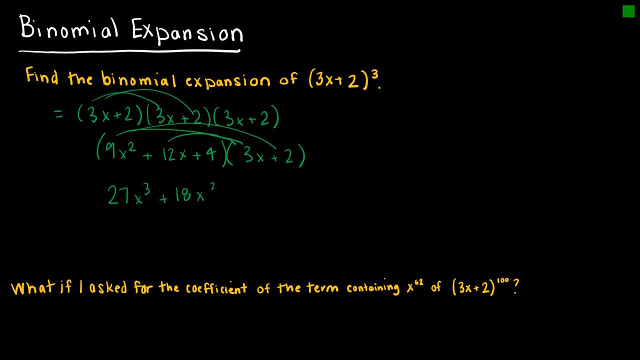 because otherwise I might make a mental mistake- 18x squared, and then 12 times 3 would be 36x squared, and then 12x times 3 would be 36x squared. So I'm going to take that times 3x plus 2 and 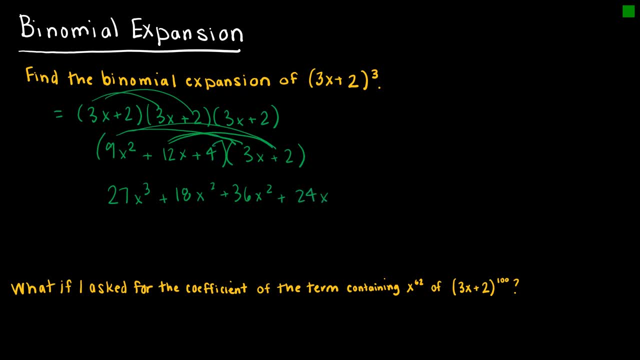 then 4 times 2 is 24x, and then 4 times 3x is 12x and 4 times 2 is 8.. And so, if I simplify all of this, I have 27x to the third. I'm combining these together to get 54x squared. I'm combining these. 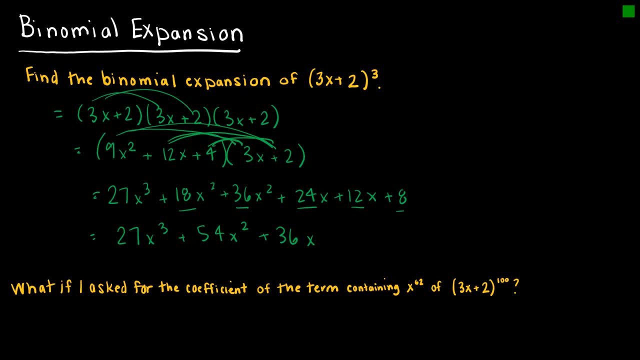 together to get 36x and then I have 8.. So if I simplify all of this, I have 27x to the third, and so that wasn't super horrible and it's something we know how to do from long, long ago. But what if I? 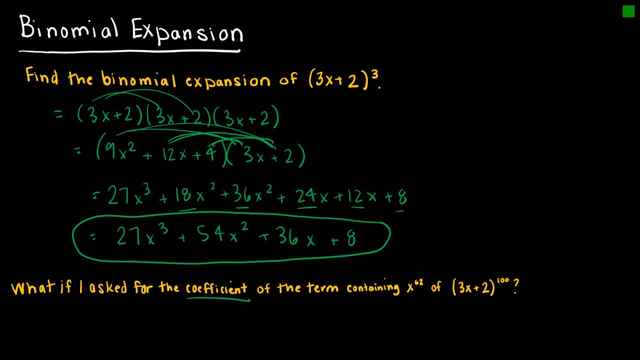 said: hey, I want to know what the coefficient is and remember coefficients like what's the number in front of the term containing x to the 62, in the expansion of this to the 100th power? Well, I don't really feel like multiplying it all out, and so we have to have a better strategy. 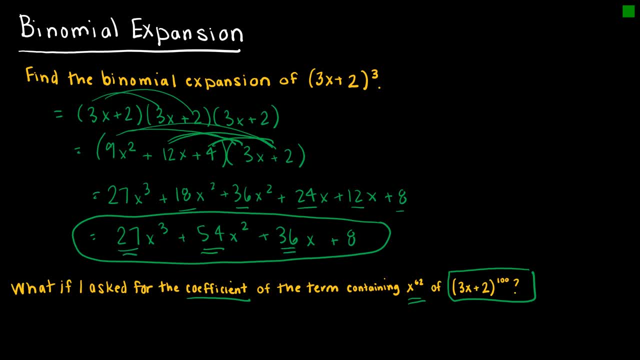 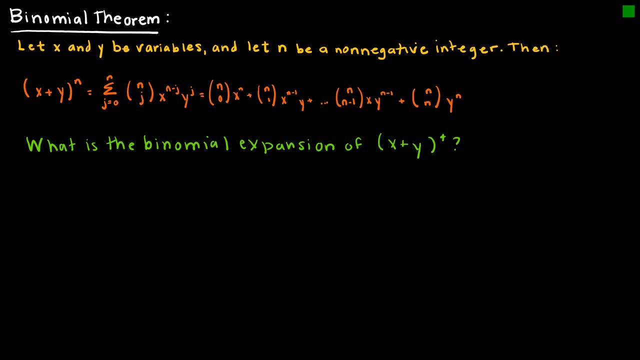 for finding the 27 or the 54 or the 36 or the 8.. So thank God we have the binomial theorem, because the binomial theorem does just that: It essentially helps us to expand our binomial without having to actually foil and then foil, and then foil and keep. 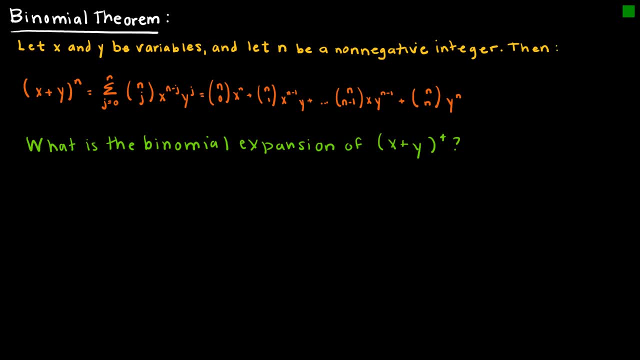 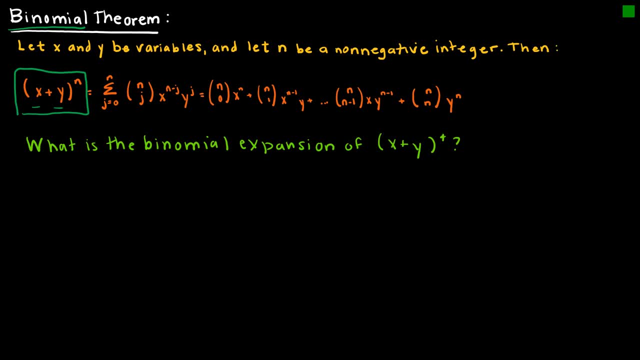 be that y is just a constant. it really doesn't matter, It's the same pattern. Essentially, what we're saying is we have the summation as j goes from 0 to n of n, choose j. so this is called a binomial coefficient, and that's really the goal here is to get those coefficients and then x to 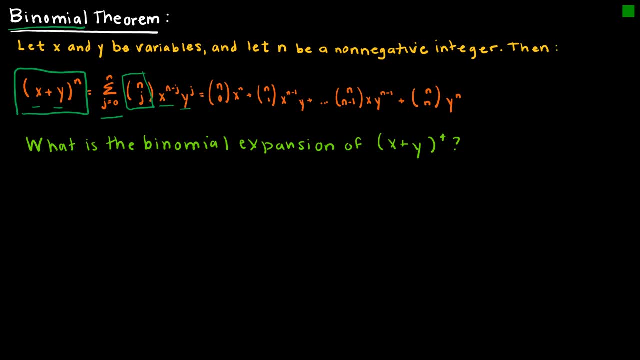 the n minus j, y to the j, And so that might not make sense to you here. I've expanded it out for you a little bit, but to me it just makes more sense when I look at an actual example example. So this one says: let's take x plus y to the fourth power, What would the binomial 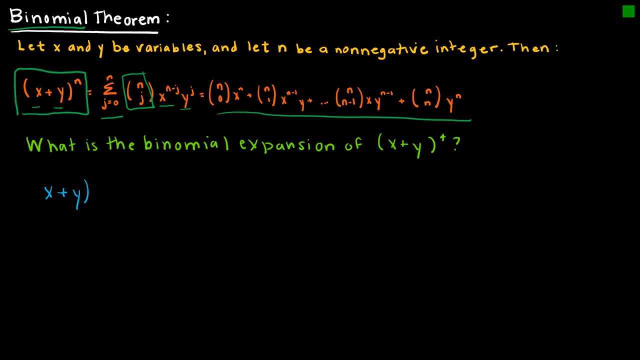 expansion be using this binomial theorem. Well, it tells me that again, I've got 4, because it's to the fourth, and I'm starting at j is 0. So 4, choose 0. and then I'm taking x to the 4 minus 0, which is 4, and y is to the 0 power, So y to the 0. Now, typically, of course, 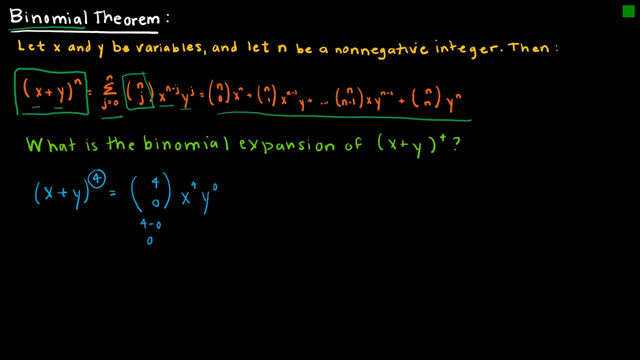 I'm not going to write y to the 0. I'm doing it now, just so you understand what's happening. Then the next term is 4. choose 1, because I'm just going to increase. So as j goes from 0 to n. 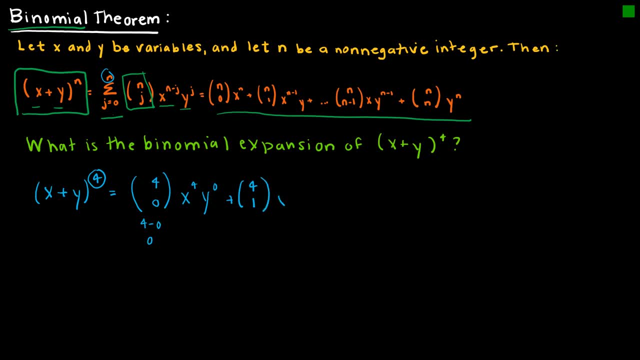 so from 0 to 4.. I'm going to keep going until I get to 4.. x is to the 4 minus 1, which is 3, and y is to the 4 minus 1.. So I'm going to keep going until I get to 4.. x is to the 4 minus 1. 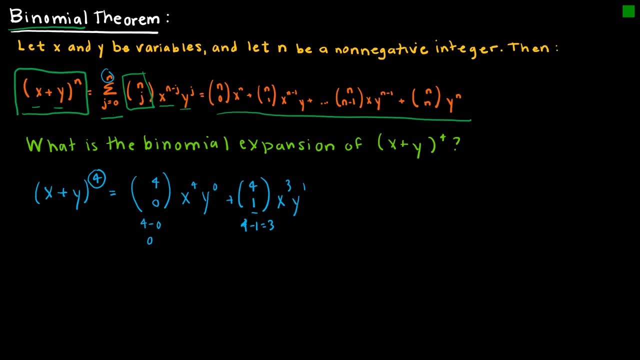 y is to the 1., And then 4 choose 2.. We can see the pattern here: x squared, y squared, 4 choose 3.. x1, y3. And 4 choose 4.. x0, y4.. Now, of course, as I said before, I'm probably not going. 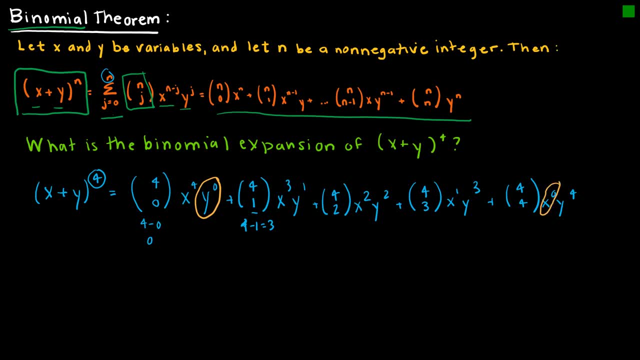 to write this one, and I'm probably not going to write this one in the future because we already know what those are. But how does this work? So I'm going to take x to the 4 minus 1.. I'm going, But how does this really help us? Because these 4 choose 0s are things that we already know how to. 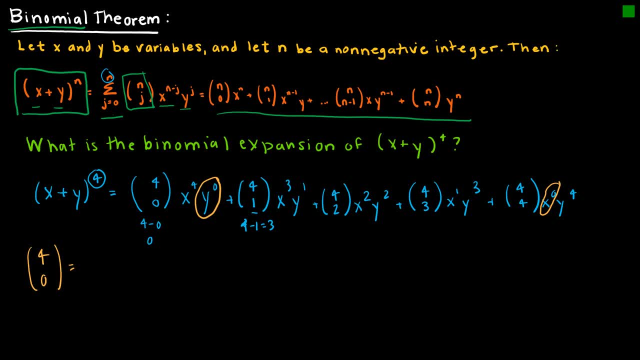 do 4 choose 0 is the same as before, when I said 4 c 0 or c 4 comma 0.. All of those things are the same. And do I already know how to find that? That tells me to take 4 factorial over 0 factorial. 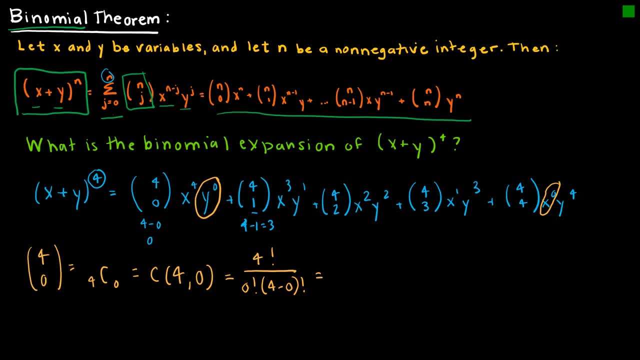 4 minus 0 factorial And that ends up with 4 factorial over 4 factorial, which is just 1.. So this coefficient is 1. And I keep doing that for each of these. So 4 choose 1 is 4.. 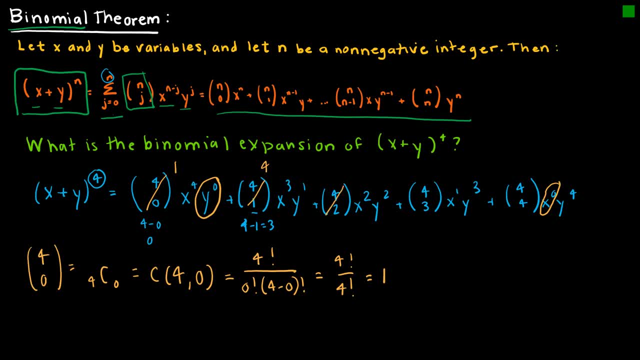 4 choose 2 is 6.. 4 choose 3 is 4.. 4 choose 4 is 1.. And so what I'm going to do is I'm going to have just found is that my answer to my expansion here is 1 x to the 4th, So I didn't even have to. 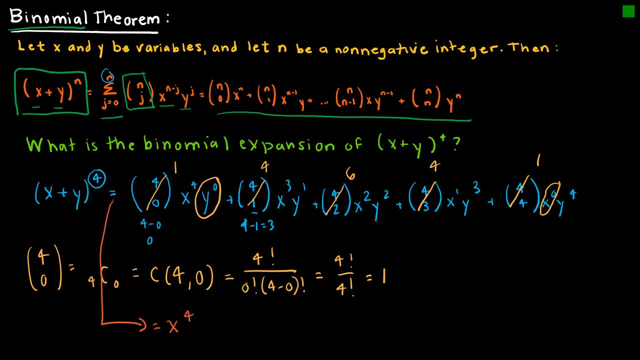 write the 1.. But it's 1 x to the 4th power And then 4 x to the 3rd, y to the 1st, And then 6 x squared y squared Plus 4 x to the 4th power. And then 4 x to the 6th power, Plus 4 x to the 3rd y to the 1st part, Plus 4 x to the 4th, Plus 4 x to the 4th Y to the same number than the previous one, which is square root squared. 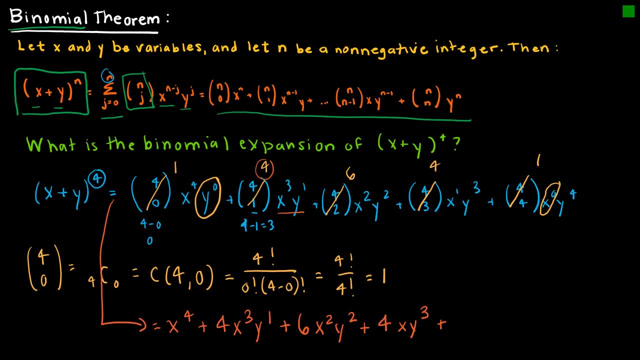 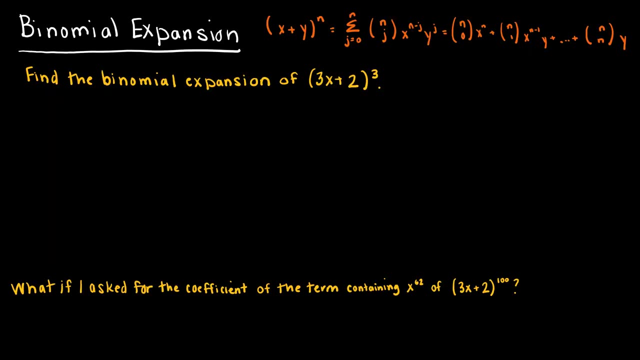 x, y cubed plus. again, I'm not going to write the one, I'm not going to write the x to the zero, so it's just y to the fourth. So I'm able to do the expansion of that without actually having to do any of the foiling. So now that we have our binomial theorem, let's take a look at how I could. 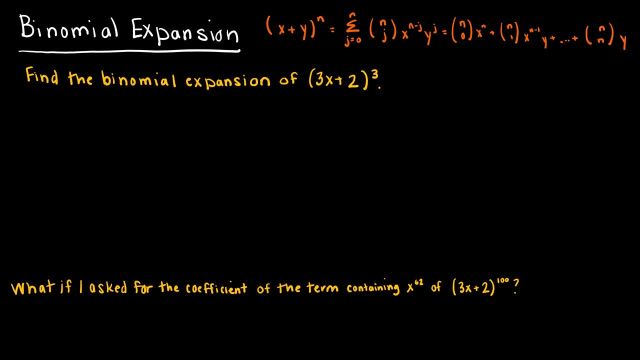 revisit this question to find the binomial expansion of 3x plus 2 quantity to the third power. So again, what I'm going to look at here is- and I encourage you to write it as a summation- the summation as j goes from 0 to 3 of 3, choose j, remember j is the one that's changing. 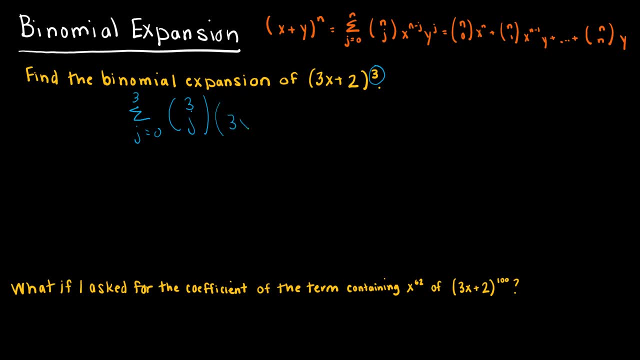 and then this is going to be 3x to the 3 minus j, and this is going to be 2 to the j. So I'm using this formula to essentially replace x with- in this case, my first term is 3x- and replace y with, in this case, 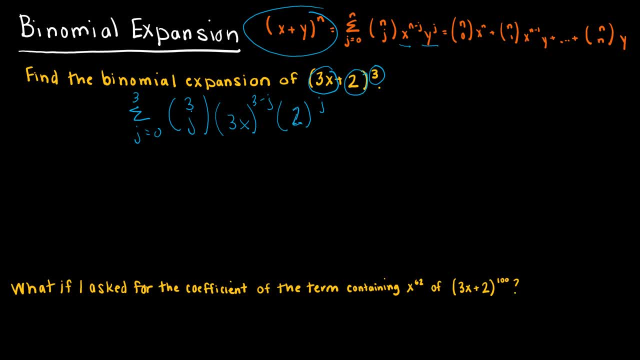 my second term is 2.. So from here, if I want the binomial expansion, I'm going to, you know, disentangle the right and left parts of the equation and I'm going to keep replacing that y with h minus 3x and I'm using that to make my second term to 200. 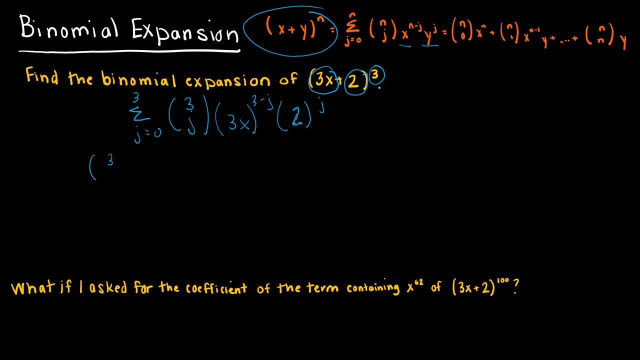 So I'm going to use this formula to essentially replace x with, in this case, my first term is 3x. use 3, choose 0, 3x to the 3 minus 0, 2 to the 0, plus, because, again, it's a summation. 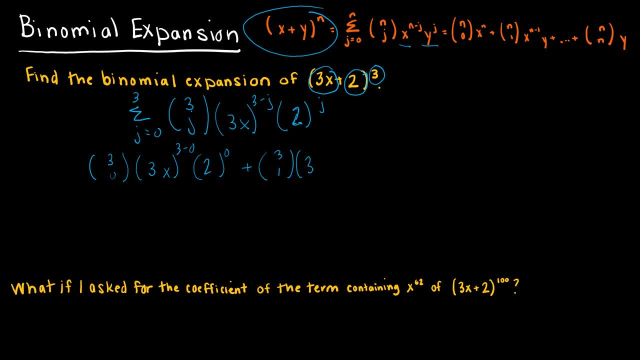 3 choose 1,, 3x to the 3 minus 1,, 2 to the first plus 3 choose 2,, 3x to the 3 minus 2, 2 to the 2, and 3 choose 3, because again that's where we stop: 3 choose 3, 3x to the 3 minus. 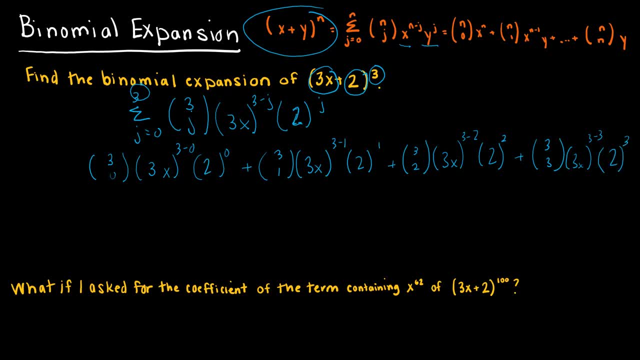 2.. So 3 choose 0, remember, is just 3 factorial over 3 minus 0 factorial, which is 3 factorial over 0 factorial and 0 factorial, if you'll recall, is 1.. So 3 factorial over 3 factorial is 1, so I have 1.. 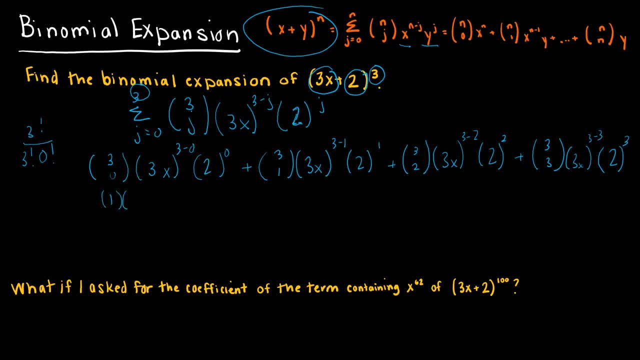 And then 3 to the 3x to the 3 minus 0,, so that's 3x to the third. so that's 3 to the third, or 27,. x to the third And then 2 to the 0 is 1.. 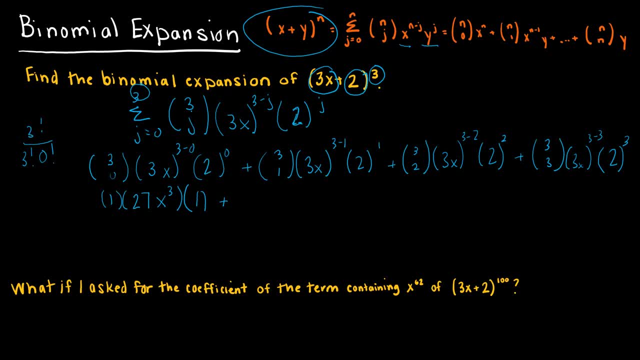 And of course I'm writing out every single step on this. you probably wouldn't do this, you wouldn't write times 1 and times 1, but I'm just doing it so that you can see where everything is coming from. 3, choose 1,. again, you can use your calculator for those binomial coefficients, or we can. 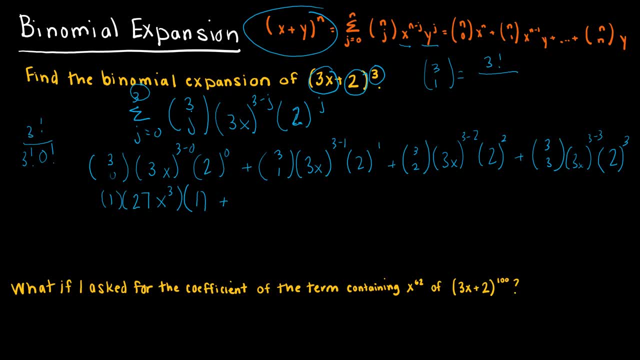 work them out. So 3 choose 1 would be 3 factorial Over 3, minus 1 factorial over 1 factorial, which gives me 3, sorry, 3 times 2 times 1, divided by 2 times 1, which is just 3.. 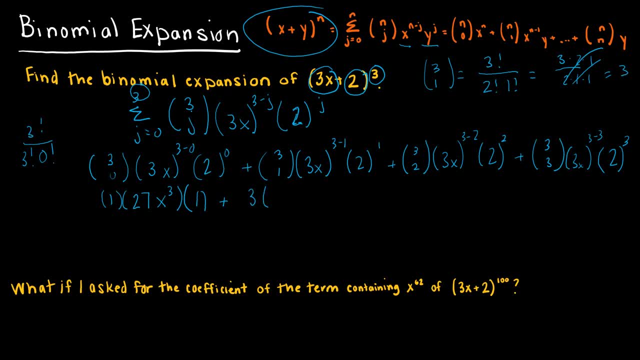 So this is 3, times 3x to the 3 minus 1 is 2,. so 3 squared is 9, and x squared is x squared, and then 2 to the first power, And then I continue. 3, choose. 2 is 3 factorial over 3 minus 2 factorial over 2 factorial. 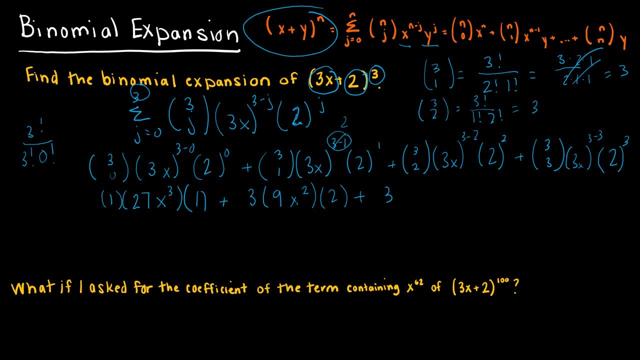 which is exactly 3, which I found before. So 3, this 3 minus 2 is 1, so that's 3 to the first, x to the first and 2 squared, which is 4.. And then we have 3 choose 3, so again, 3 choose 3.. 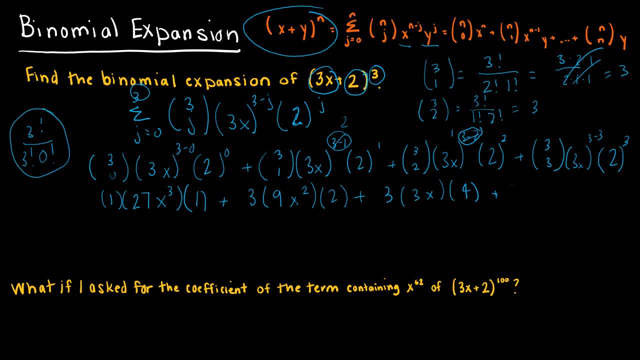 I'm going to look exactly like this one and that's going to give me 1,, 3x to the 3 minus 3,, which is 0,, so 3 to the 0 is 1, and then x to the 0,, which is also 1,, which you don't. 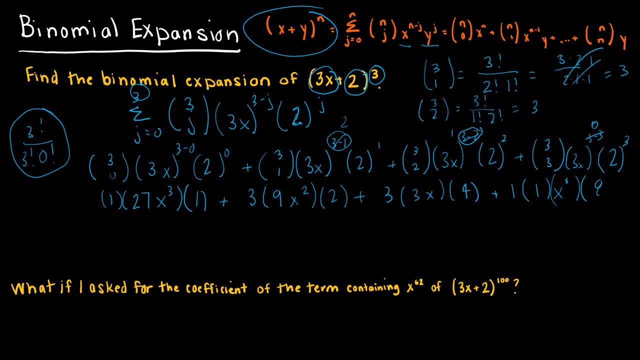 even have to write again, and then 2 to the third, which is 8.. So now I'm just going to do the math. So 1 times 27, times 1 is obviously 27x cubed, And then we have 3 times 9, which is 27,, times 2,, which is 54x squared, and then we 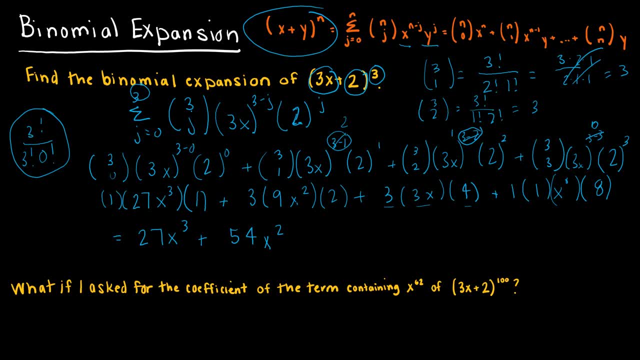 have 3 times 3 times 4,, so 9 times 4, or 36x, and then 1 times 1 times 1 times 8, which is 8.. And if you'll recall, this is exactly what we found before when we did it by hand. 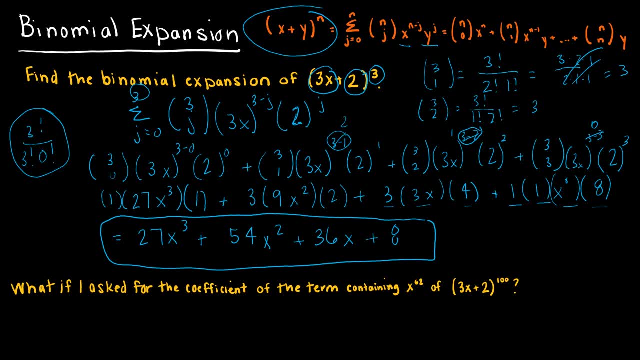 Now you might be saying, okay, hold on, That was more work. And for a question like this one it you know it's give or take more work, But for a question like this one, obviously I don't want to do the expansion. 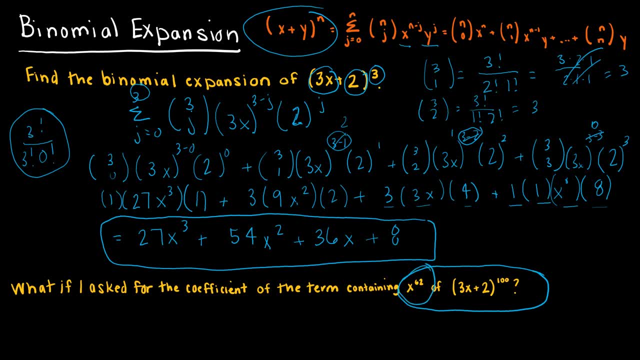 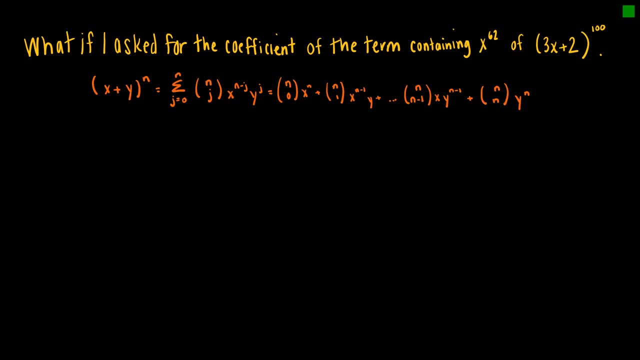 So now let's take a look at finding the coefficient of x to the 62nd. So let's go back to my original question that I didn't want to have to foil out by hand. What if I asked for the coefficient of the term containing x to the 62?? 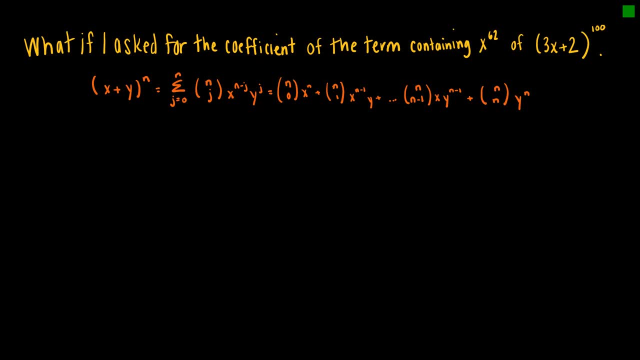 What if I asked for the coefficient of 3x plus 2 to the 100?? So the first thing I should think about is again- and I've rewritten this binomial theorem for you, but it's okay to write this as the summation- 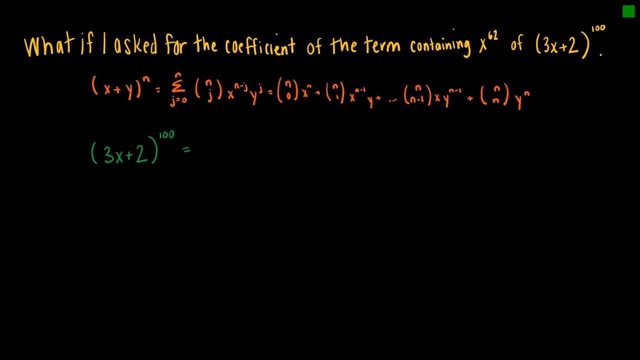 And in fact I encourage you to, because to me that helps it make sense when I'm trying to find a specific term. This tells me that I'm finding the summation as j goes from 0 to 100 of 100. choose j and. 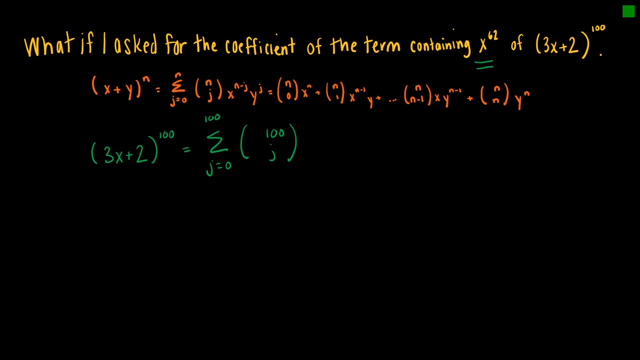 again, that's the summation, And I'm trying to find the summation And I'm trying to find the summation And I'm trying to find the summation. j is that value that is going to change. And then it's going to be, instead of just x to the n minus j, it's going to be 3x to 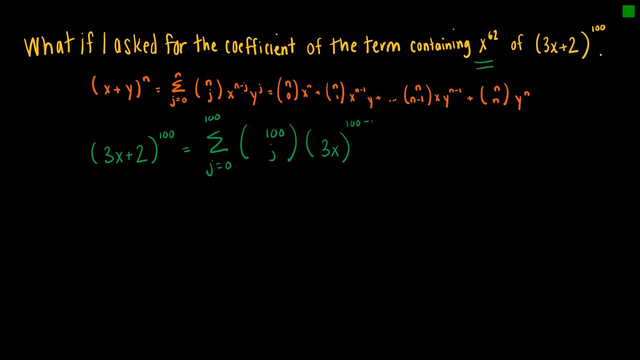 the n minus j, So 100 minus j, because n is 100, obviously. And then, instead of just y to the j, I don't actually have a y, it's just 2, and it's 2 to the j. 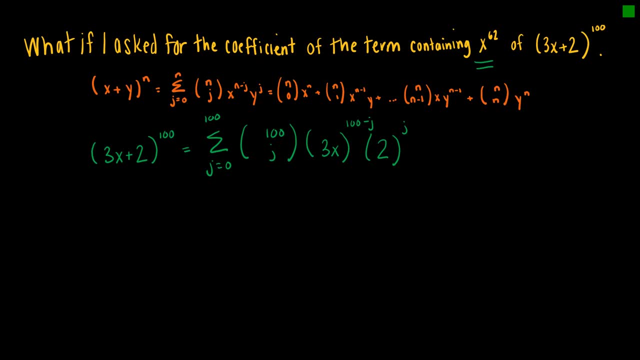 So this is how I would rewrite. I would rewrite it using the binomial theorem as a summation. So what did that do for me? Well, I'm trying to find the coefficient where x has a coefficient of 62. And so I want to say that 100 minus j has to be 62. 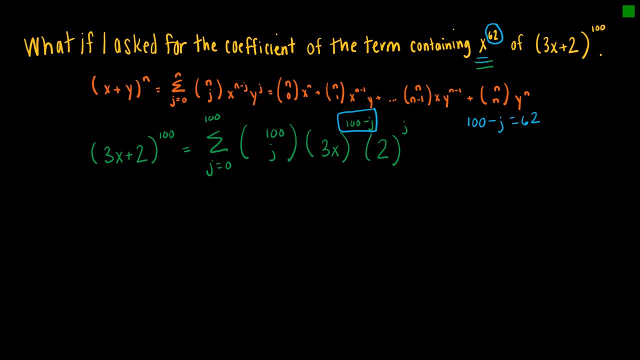 How do I know that? Because I want x to have an exponent of 62, and this is the term with x on it, So 100.. So 100 minus j must be 62. So j must be 38.. Again, now I'm going to take what I know here and I'm going to use j of 38 to help me find. 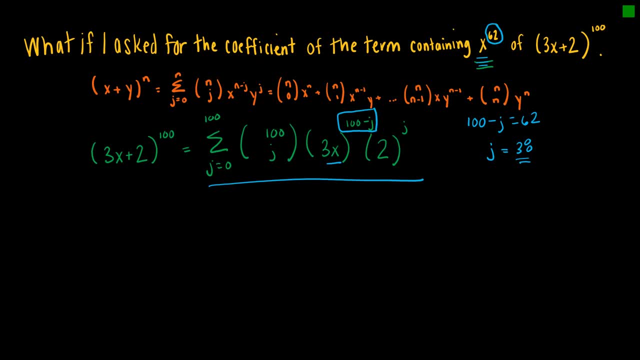 the solution. So this tells me that the coefficient for x to the 62nd is 100. choose j, So 100.. Choose 68.. 3x to the 100 minus j, which was 62, because that's what I wanted, right. 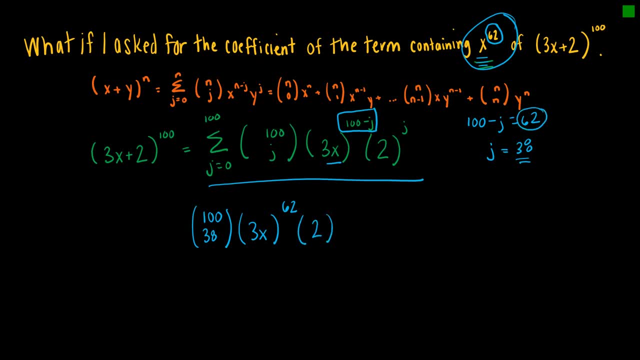 62. And 2 to the j, which is 38. So that's going to be my solution, And now I just have to do the math. Like I already have it set up correctly. This tells me I'm taking 100 factorial over 38 factorial. 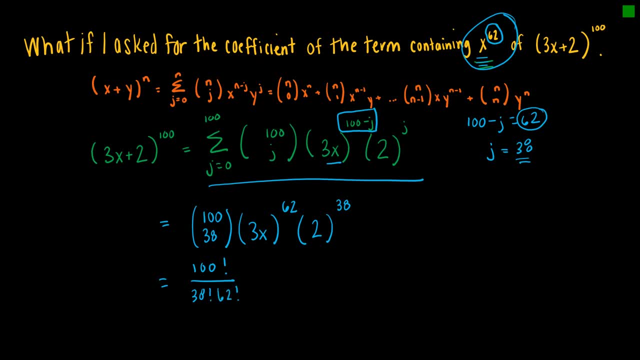 62 factorial, and then this is obviously 3 to the 62nd and this is 2 to the 38.. And you might be asking: hold on, what happened to x? Do I really care about x? Well, I know that when I'm done, this is the number in front of x to the 62, but I'm really 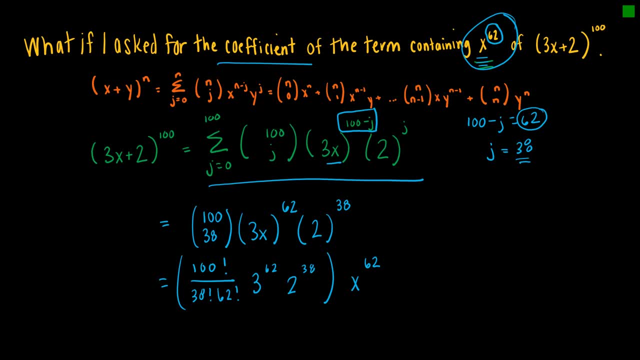 just looking for the coefficient, So I don't need to keep that x to the 62 on there. I'm just finding the coefficient. Now could I actually go ahead and compute this solution? I could, but this is going to be astronomical. 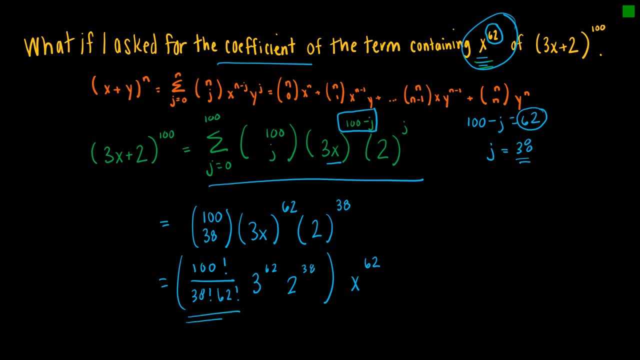 I mean, even just finding this value is my calculator is not going to compute it because it's so many numbers that it just doesn't make sense. So again, as I had stated before, quite often in combinatorics we just leave our answer. 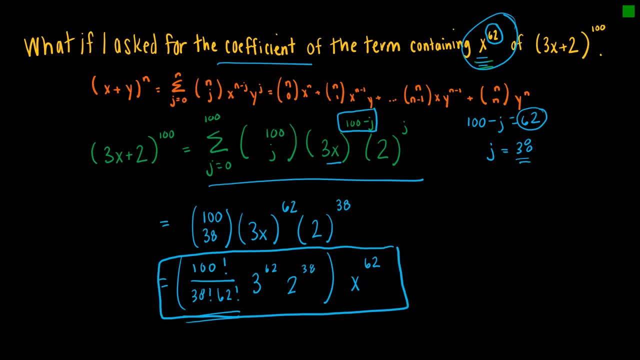 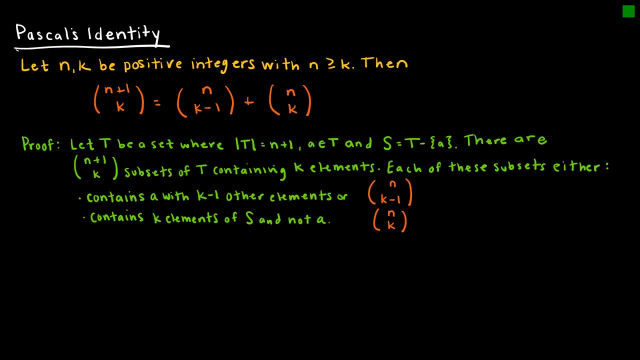 in this kind of format. And so what would be the coefficient? It would be just this part right here. This would be my solution to that question. The last thing I want to talk to you about this week is Pascal's identity and Pascal's. 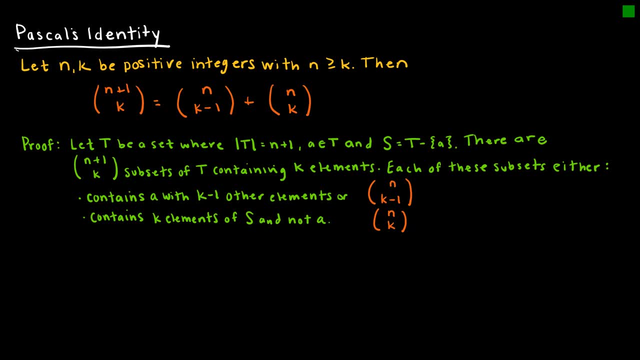 triangle, which are obviously related. And Pascal's identity says: if n and k are positive integers with n greater than or equal to k, then n plus 1- choose k- is equal to n. choose k minus 1 plus n- choose k. And again, this is just an identity that you're going to use literally all of the time in 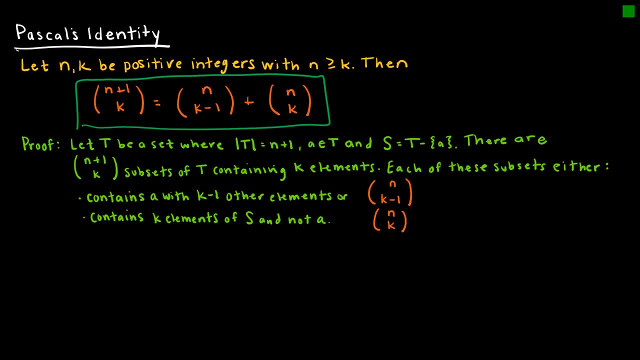 combinatorics. We're going to use it. You'll need to know it, But for now again, it's just a nice introduction And I've included the proof here so you can kind of see or understand why this identity works. 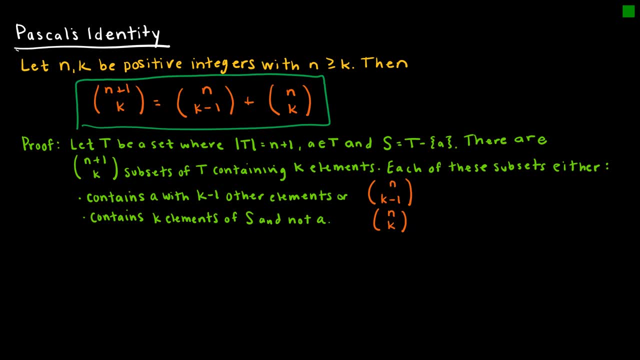 So we're going to say: let t be a set where the number of elements in the set of t is n plus 1.. So we have n plus 1 elements And a is in the set t and s And a is t minus the element a. 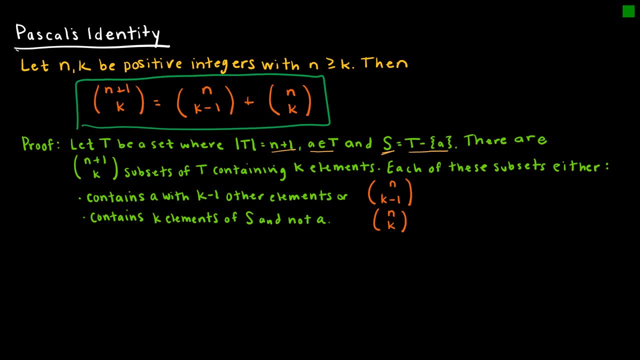 So essentially we're saying there are n plus 1. choose k subsets of t that contain k elements And each of those subsets- either- So this is equal to- either contains a with k minus 1 other elements, or it doesn't contain a. 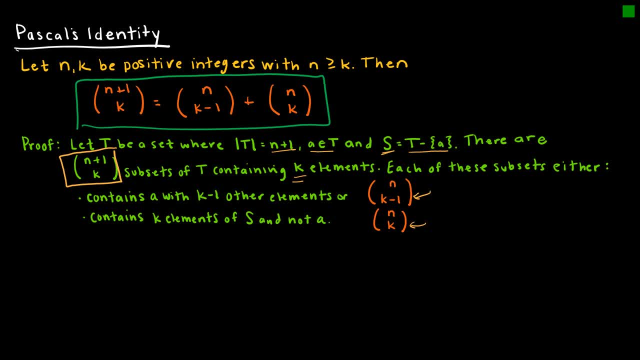 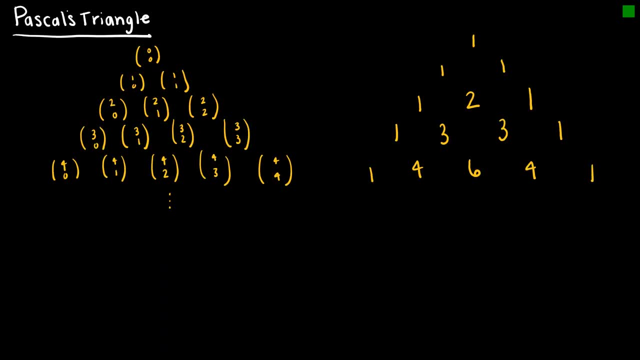 And therefore there's k. That's just one of the elements in there, So that's just a way to show that the two sides are equal to one another. So why does this matter? Well, because Pascal's triangle is based on that identity. 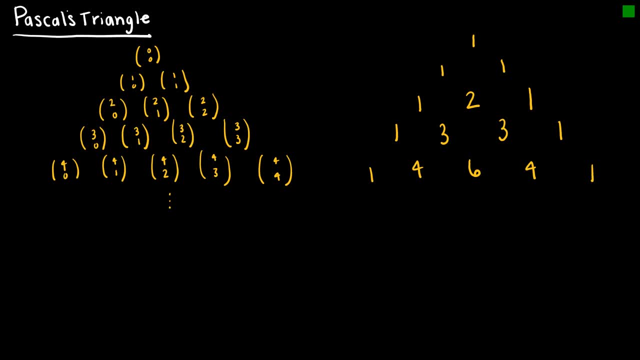 And Pascal's triangle. if you can see, this is just 0 choose 0, and then 1 choose 0, and then 1 choose 1, and then 2 choose 0,, 2 choose 1,, 2 choose 2.. 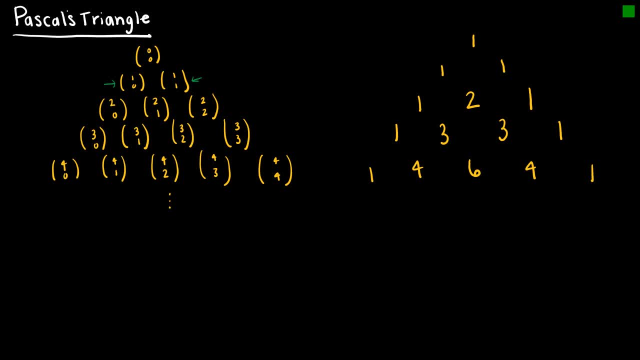 These are the rows of Pascal's triangle. Well, what does that do for me? Pascal's triangle triangle is, if you'll remember, we worked through x plus y to the fourth and we found the coefficients. we we did all of this using the binomial theorem. we said that was x to the fourth plus four x to. 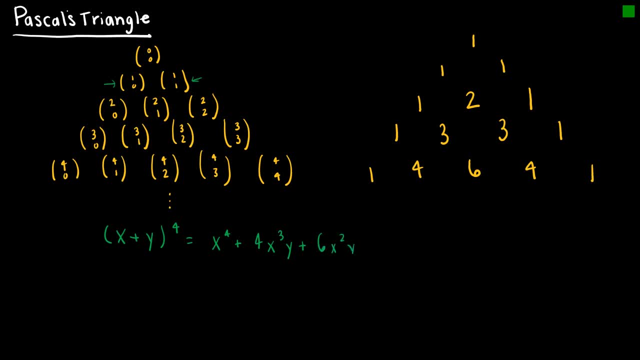 the third, y plus six, x squared, y squared plus four, x, y cubed plus y to the fourth. so we just did this together a little while ago. so pascal's triangle says: hey, those numbers one and four and six and four and one can be found in this row of pascal's triangle: one and four and six and four and one. 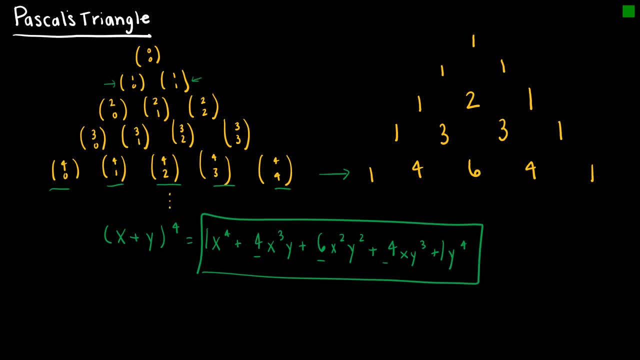 so why does pascal's identity matter then? where does that come from? well, pascal's identity says: if you've got two consecutive elements, you can add those together to get the next value of your pascal's triangle. so three plus three is six, and one plus three is four and you get the.